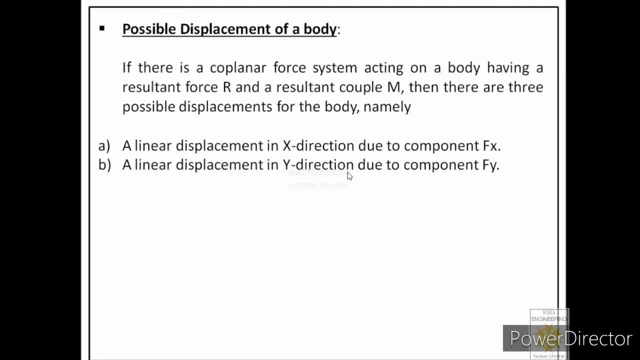 There can be a linear displacement of the body in y direction due to the component FY of all the forces and there can be a rotation due to resultant couple M of all the forces. so these are the three possible displacements of a body when it is under the action of a force system. 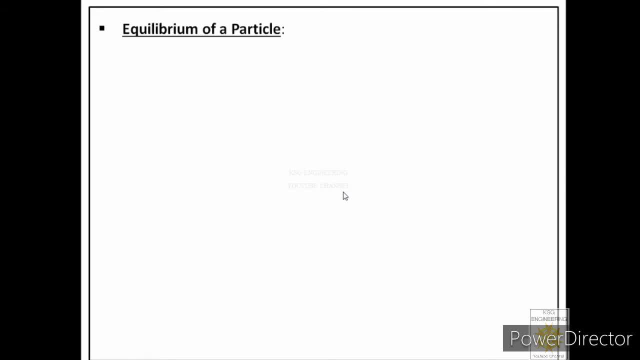 now let us relate that with the equilibrium of a particle. so in the first slide we said that if the net effect of all the forces- that is, force system- acting on the body is zero, then the state of motion of the body will remain unchanged. now let us relate that to the possible displacements of the body under 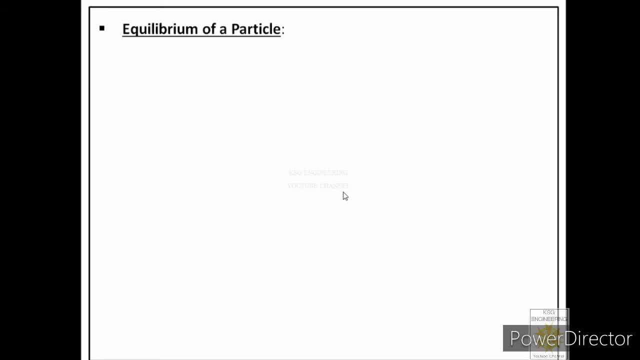 the action of the forces, then we will find that in equilibrium of a particle, the sum of all the forces acting on the body in x direction is zero. therefore, the component effects of all the forces acting in the force system must be equal to zero. similarly, the sum of all the 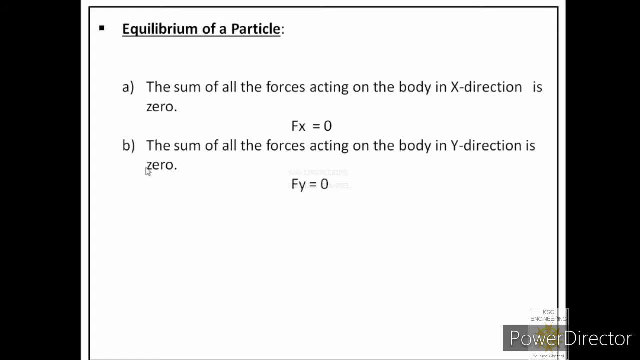 forces acting on the body in y direction is zero. that means FY should be equal to zero and there should not be any rotation of the body as well. that means the moment, because of all the forces acting on the body, is zero. so we have concluded that if a body is in equilibrium under the action of a force, 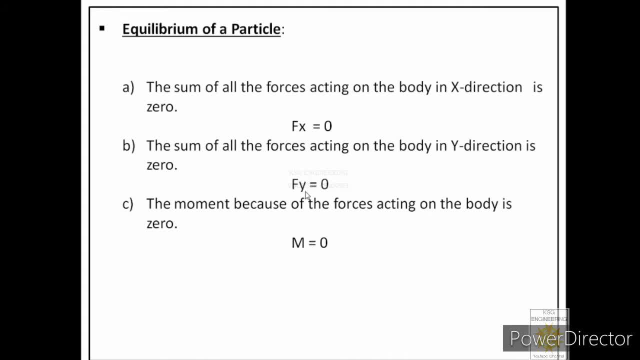 system, then all these three equations are applicable on that body. so we call these three equations as equations of equilibrium. that means if number of forces are acting on a body and body is in equilibrium, that means if we will add the components of those forces acting in x direction, their sum has to be zero. 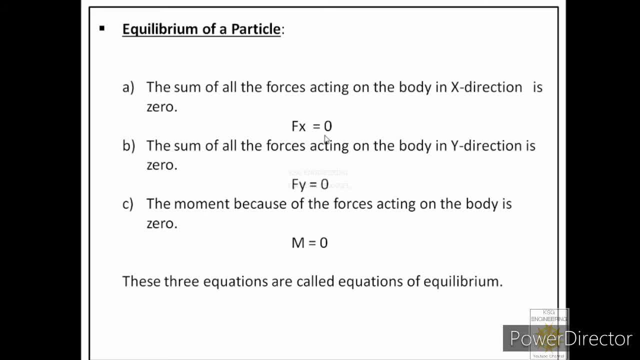 because body is not moving in x direction. similarly, the sum of the components of all the forces acting along the y direction must be equal to 0, because body is also not moving in y direction. Similarly, the moment or the couple because of those forces must be equal to 0, because body 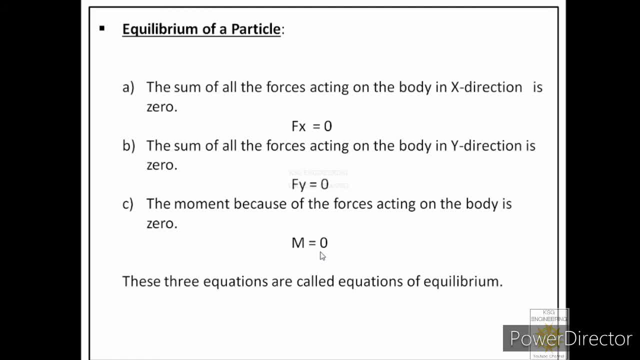 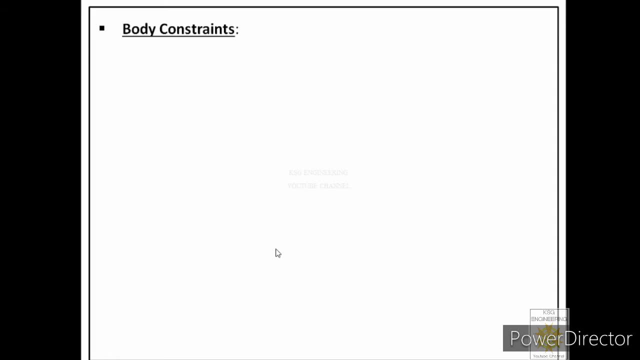 is not rotating. So we will make use of these three equations in the numericals related to equilibrium of a particle. Now we'll talk about body constraints. A body constraint is a contrived sport or force provided such that the body remains in equilibrium. Constraints provide reactive forces and or couples. 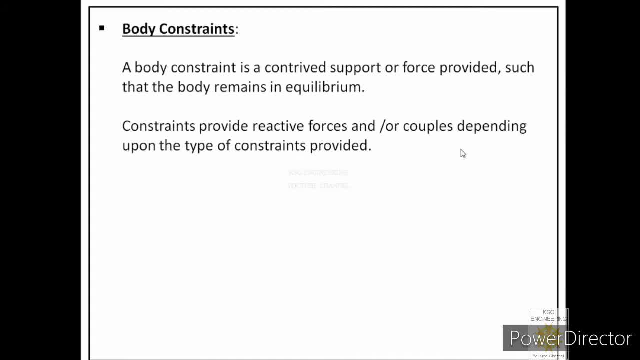 depending upon the type of constraints provided. So let us understand this through an example. What are body constraints? If you have to give example of body constraints, then photograph hanging on a nail is the best example. So let us see how. Suppose our photograph is hanging on a nail and 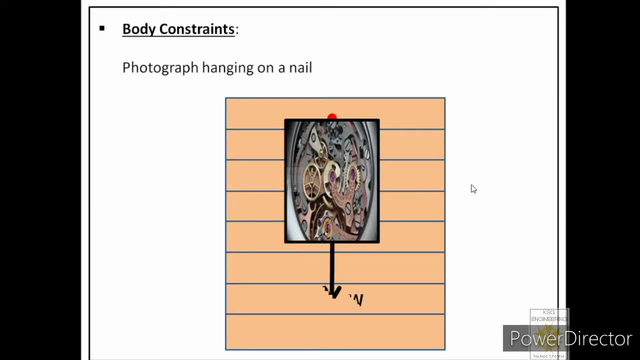 let us see what is happening over here. The weight of the photograph is acting in downward direction, but still it is in equilibrium. Why? Because there is one constraint, provided by the nail, that is the reaction which acts in opposite direction, and this reaction is equal to weight of the photograph. So the constraint. 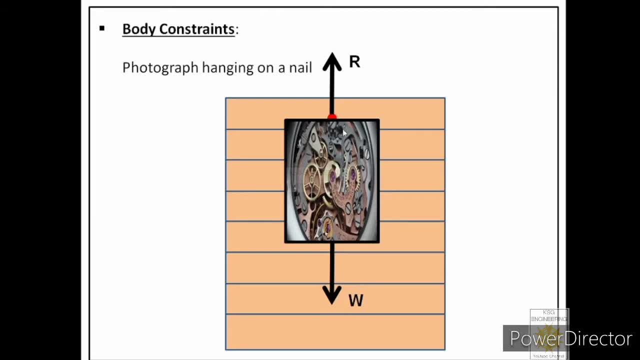 provided by this nail helps this particular body to remain in equilibrium. So over here we will say that nail is acting as a body constraint which provides a constraint to the motion of the photograph in vertical direction. So we can say the reaction provided by the nail is equal to weight of the photograph. Now we will see the constraints provided by. 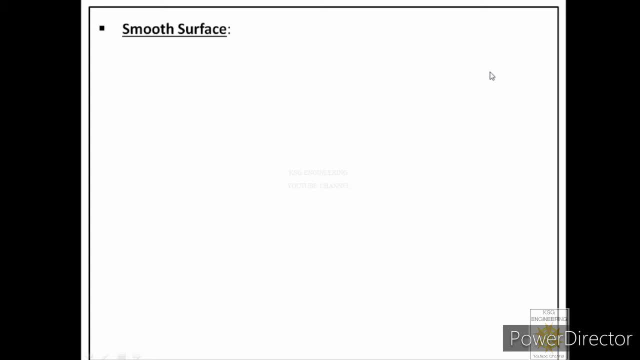 a different body constraint. So we can say that nail is acting as a body constraint. Let us first talk about smooth surface. Suppose we have a smooth surface and on that surface body is placed. Now we know, for every body there can be three types of motions. Either 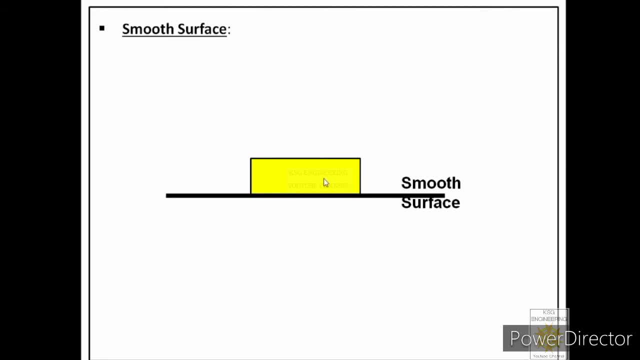 body can move along x direction, or body can move in y direction, or body can rotate. So if we will talk about smooth surface, It will provide only one body. constraint means smooth surface will not allow the motion of the body in y direction. The weight of the body is balanced by the reaction provided. 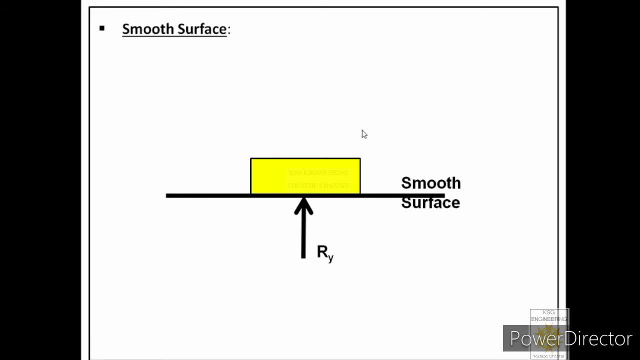 by the smooth surface, But the body can move along the surface that is, in x direction and body can rotate as well. So what we have learned? smooth surface can provide only one body constraint: The body can move in y direction or body can rotate as well. So if we will talk about heavy 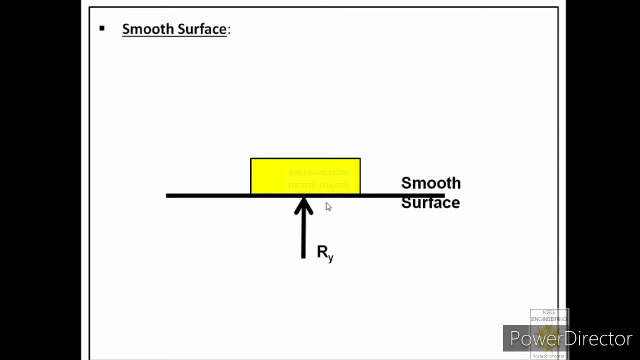 and tight motion which acts at 90 degrees to the surface, or we can say normal to the surface. Now let us talk about rough surface. Suppose we have rough surface and on that surface body is placed. Now again, we know that there can be three possible displacements of the. 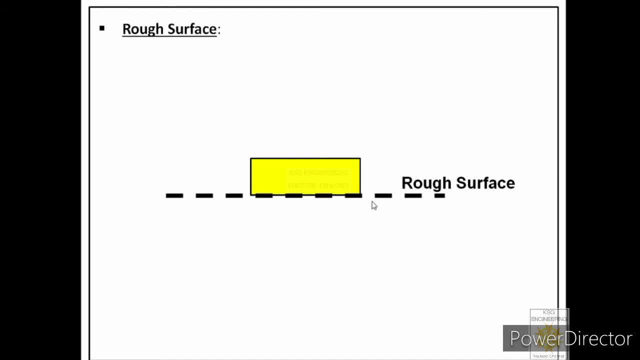 body. body can move in x direction or along the surface. we can also say the movement will be gentle. so just imagine this is the position of the body. can move in y direction. that is normal to the surface. or body can rotate, but rough surface provides two types of body constraints. first, body constraint. 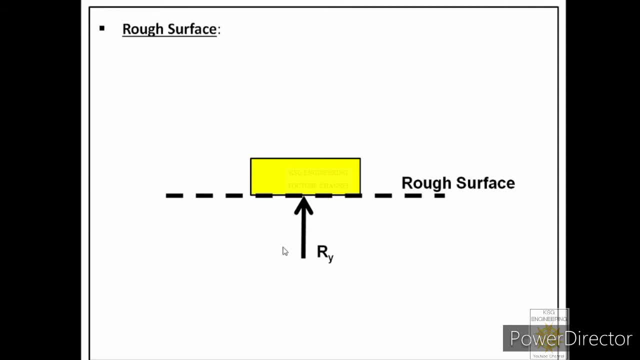 will be normal to the surface. this body constraint will restrict the motion of the body in y direction, or we can say normal to the surface. rough surface will also provide one more body constraint and this will be along the surface and this will not allow the movement of the body along the surface. but body can. 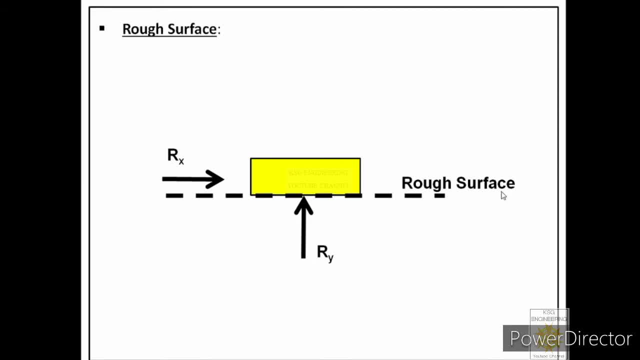 rotate. so we have learned. rough surface provides two types of body constraints: one normal to the surface, one normal to the surface. let us learn about the next body constraint, that is, roller support. roller support is used to support the bodies. normally we use such supports in bridges that we will see. 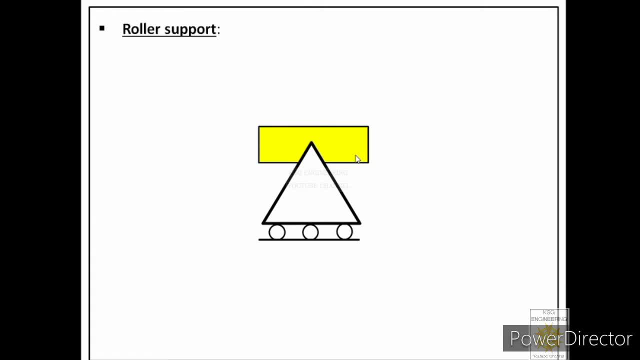 when we will take some problems on trusses. now let us see what type of body constraints a roller support can provide. you can see in this picture this is a roller. it has rollers at the bottom and at the top. it supports the body. now body is supported by this roller support and to body, roller support provides only one. 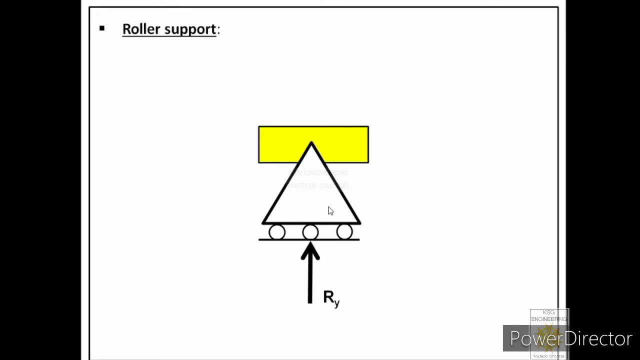 constraint that is normal to its surface means it restricts the motion of the body normal to the surface. but body can move along the surface. our body can rotate as well. so roller supports provide only one type of body constraint that is normal to the surface. next we will talk about rocker support. so these 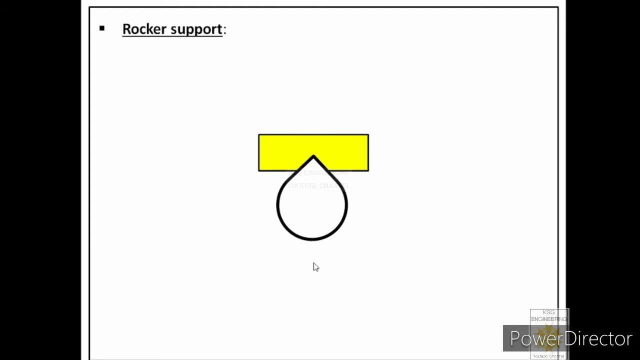 supports are also used to support the bodies. so in rocker support we have a curved surface at the bottom and like roller supports, these supports also give only one type of body constraint, that is, they don't allow the motion of the body normal to the surface. but body can move along the surface. our body can rotate as. 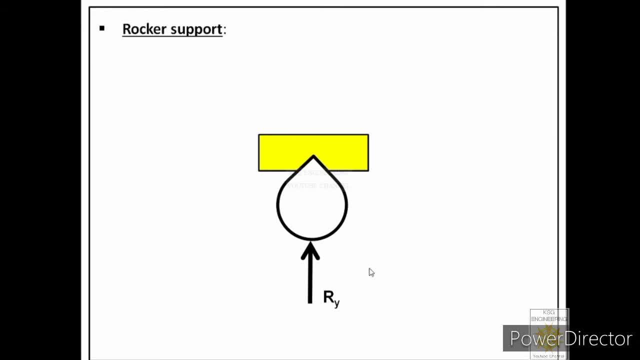 well. so remember, rocker supports provide only one type of body constraint that is normal to surface. next we will talk about hinge support. it is also known as pin support. this is a hinged support. it also supports bodies. hinged support restricts two types of motions of the body. body cannot move along the surface body. 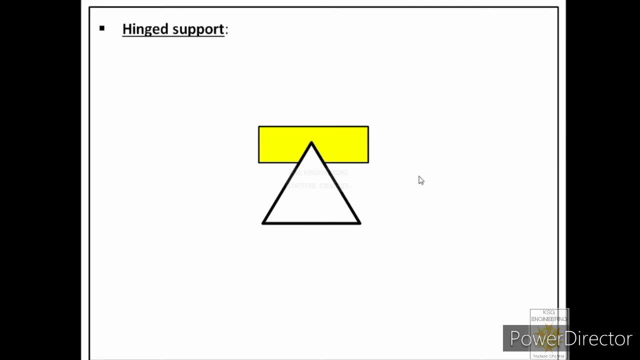 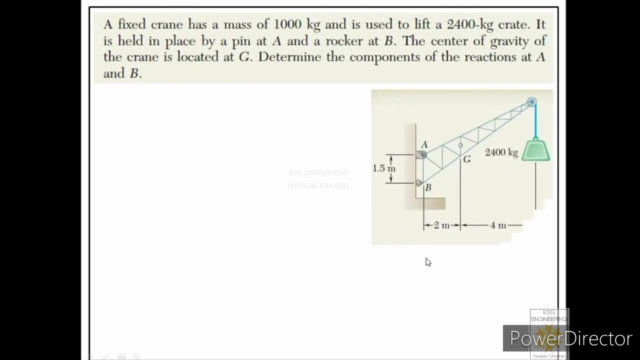 cannot move, normal to the surface, but body can rotate. therefore, hinged support provides two body constraints: one normal to the surface, one along the surface, now based on the learning of equilibrium of a particle or body, and the body constraints provided by different supports. let us solve few. 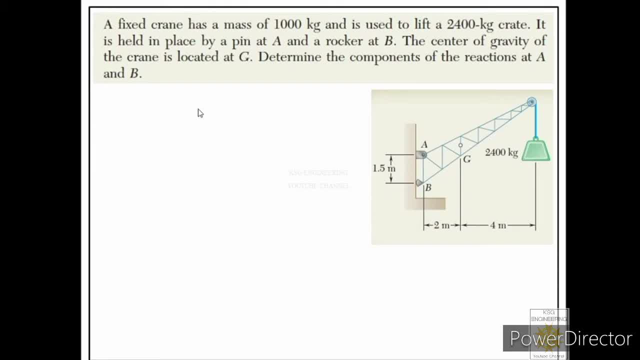 numericals. let us start with the first numerical. a fixed crane has a mass of 1,000 kilogram and is used to lift a 2400 kilogram crate. it is held in place by a pin at A and a rocker at B, the center of 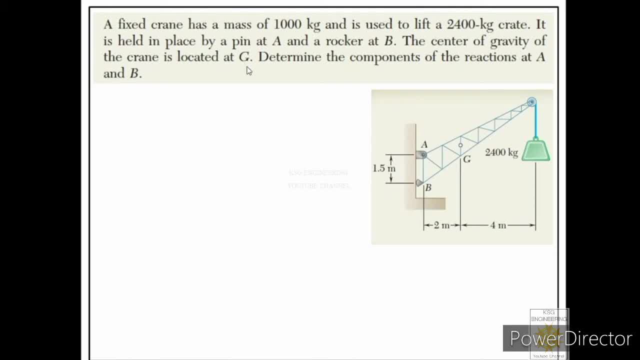 gravity of the crane is located at G, determine the components of the reactions at A and B. so one diagram is given to us. let us understand the problem through this diagram. so there is one fixed grain and the mass of that fixed grain is 1000 kilogram and it is used to lift a crate. 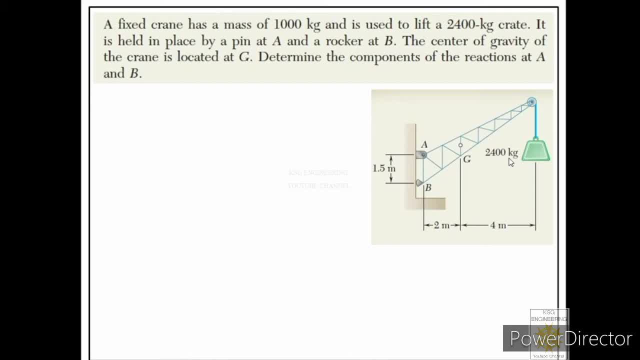 whose mass is 2400 kilogram, and we have two sports. one is pin support, or we can say hinge this support at end a and a rocker support at and B, and the center of gravity of the crane is labeled at G. now we are asked to find the components of 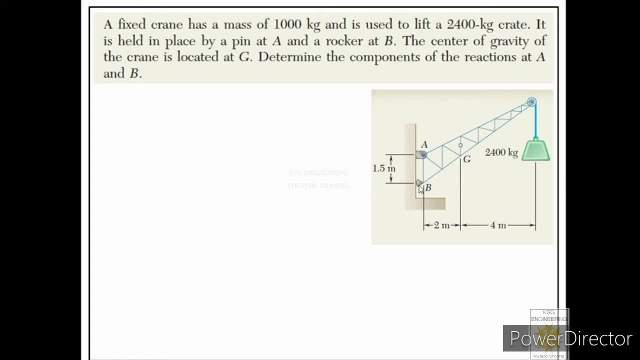 the reactions at A and B. so in order to solve this problem, first of all we have to draw the free body. so in order to draw the free body, what we will do, we will draw whatever is given in this diagram, first on the notebook, then after that we will label active forces, reactive forces and weight of the body. 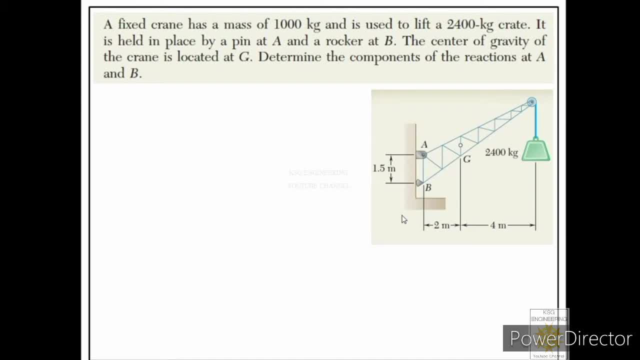 we will show their direction and magnitudes. so let us start with the reactive forces first. now we know we have two types of supports over here. one is pin support or hinged support. the other one is labeled as rocker support. in this case we have two types of supports. one is pin support or hinged support. the other one is labeled as rocker support. in 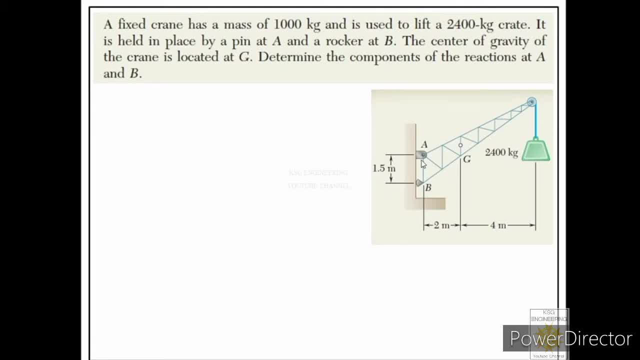 the previous slides we have learned that pin support provides two types of body constraints. it don't allow the motion of the body along the surface and normal to the surface. this is the surface of pin support. it means we can show one body constraint normal to the surface and we can show other body constraint along the surface. 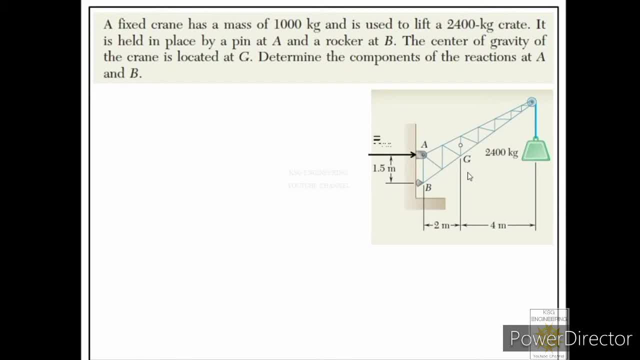 so let me show those two body constraints now. so this is normal to the surface and this is along the surface. over here we have to understand one very important point. initially, we don't know the direction of these two reactions, so we have to assume their direction. I have assumed that this particular direction 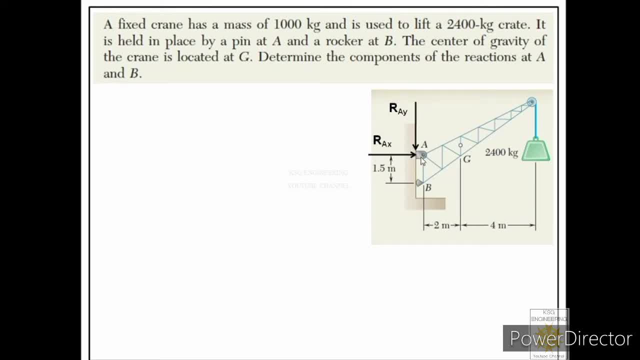 is acting towards right for the normal constraint and this direction is acting in downward direction for the constraint along the normal. when we will solve for these two constraints and if we get positive answer for this constraint, that is RAX, and the other constraint, that is RAY, then positive answer means that 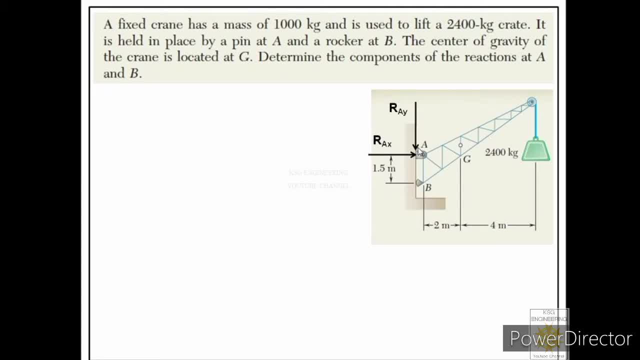 whatever assumptions we have made regarding the directions of these two reactions, then that assumption is correct. but suppose I got negative answer for this normal constraint. then that negative answer means that assumption which I took at the start for this particular constraint is wrong. it will actually act towards left. so 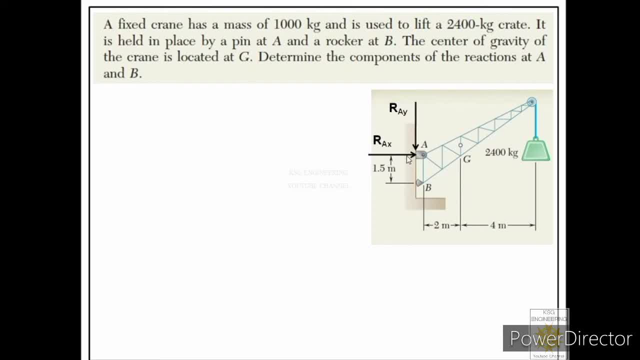 this you should keep in your mind when we level the reactions provided by a particular support. at the start we don't know their directions, so we just assume their directions at the start of the numerical. we solve those reactions. we get their numerical value if the magnitude of those reactions remains. 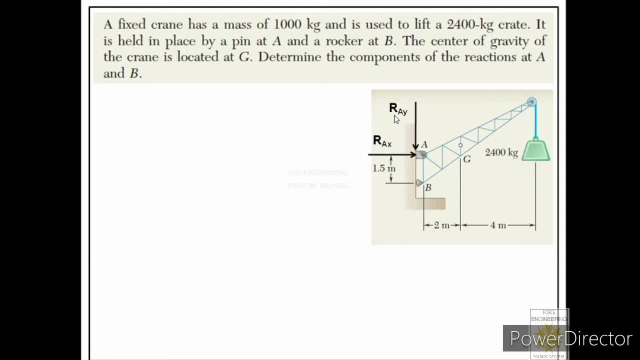 positive in the calculations, then we come to know that the directions which we have assumed at the start of the numerical are correct. otherwise we have to reverse those directions at the end of the answer. okay, so over here I have labeled this particular normal constraint as a reaction at a in X. 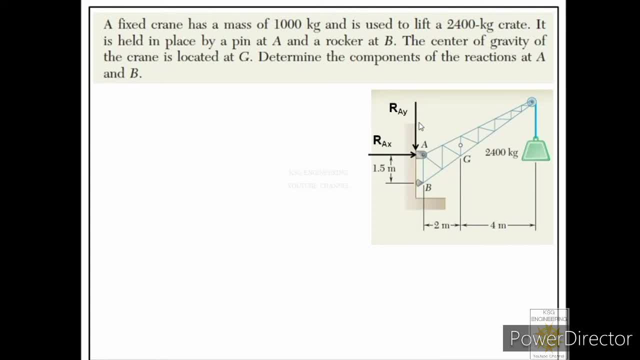 direction. I have labeled this constraint as a reaction at a in Y direction. next is rocker support. in the previous slides we learned that rocker support provides only one type of constraint: it don't allow the body to move normal to the surface. so let us show that constraint. so we have labeled one constraint: normal to the surface means. 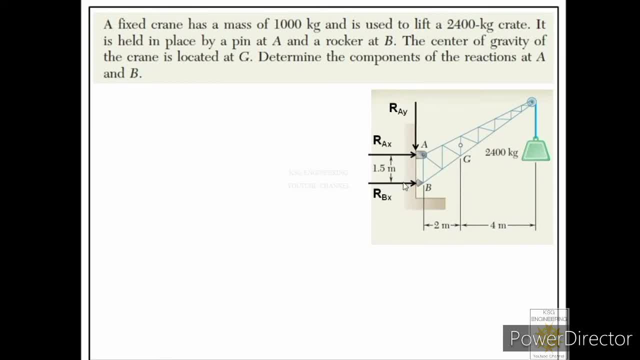 at 90 degrees to the surface of rocker support and the point mentioned for rocker support is B, so we have labeled it as reaction at B. but the direction is X direction, so reaction at B in X direction. so for this reaction also, we don't know its direction at the start, so we have just assumed that it is acting. 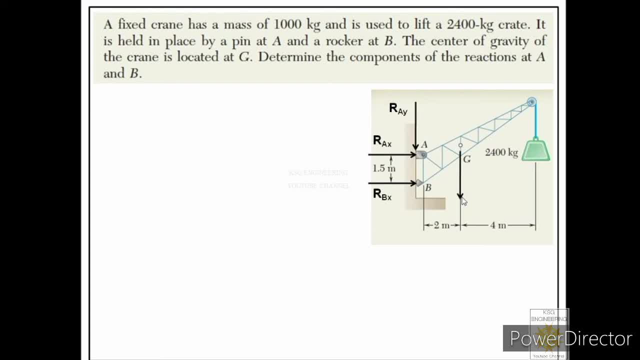 towards right. after that we will label the weight of the isolated body. so isolated body over here is crane. so weight in the problem is given as 1000 kilogram. so let us label it in downward direction. then we will label other external forces. so other external force is the weight of the crate. it will. 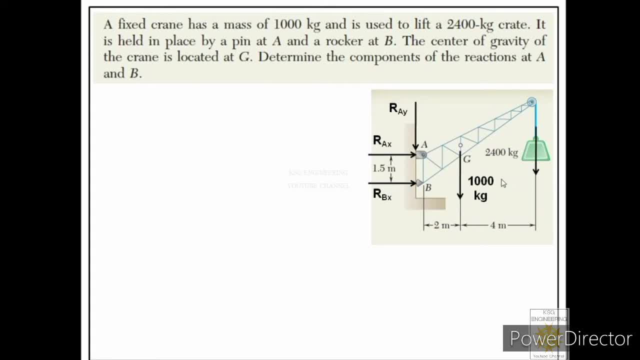 also act in downward direction. now remember, over here we have labeled thousand kilogram. so this is not weight, this is mass. so in the calculations we have to multiply it by 9.81 to get the weight of the isolated body. that is similarly, 2400 kilogram is mass of the crate. but in the calculations, when we 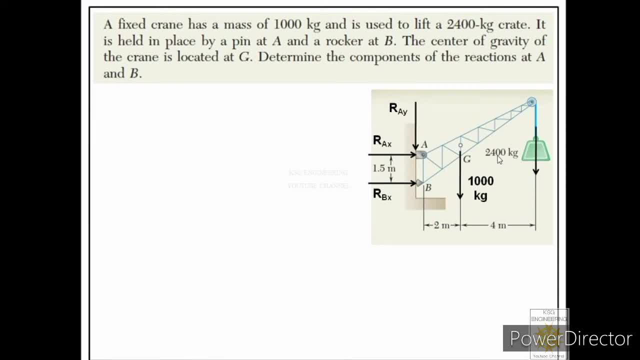 will consider the weight of the crate. we have to multiply 2400 by 9.81. now let us start the calculations. now we have to apply three equations of a kilogram over here. in this particular problem, we have five forces. fine, and we can say that in this force system there are five forces acting, and we know that for 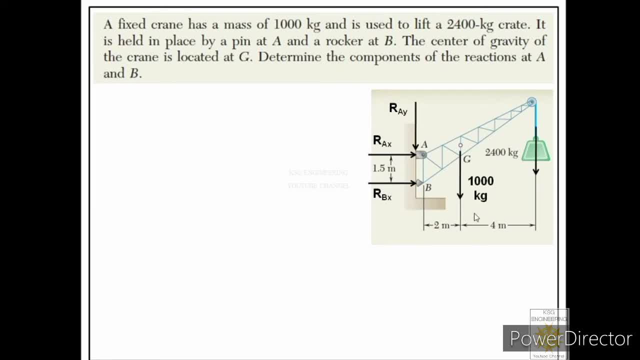 this particular position shown, the body or the system is in equilibrium. so that means the components of all the forces acting along X direction. their sum must be 0. that is summation FX is equal to 0. similarly, the components of all the forces acting along Y direction. that sum must be equal to 0. that is summation FY. 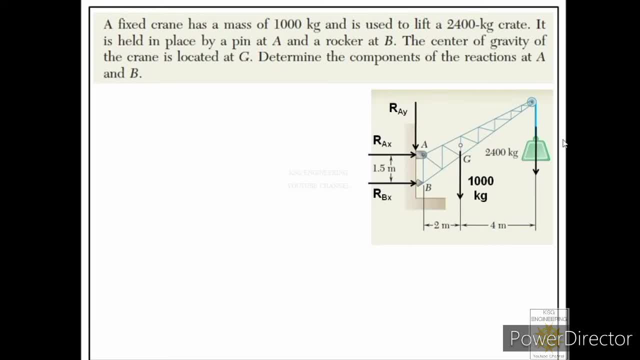 equal to 0, then the moment, because of all the forces about any particular point in the free body, must be 0, because body is not a rotating body, is in equilibrium. so we will use all those three equations to solve for the unknowns. so what are the unknowns for us? we have RAYRAX and RBX and these three we have. 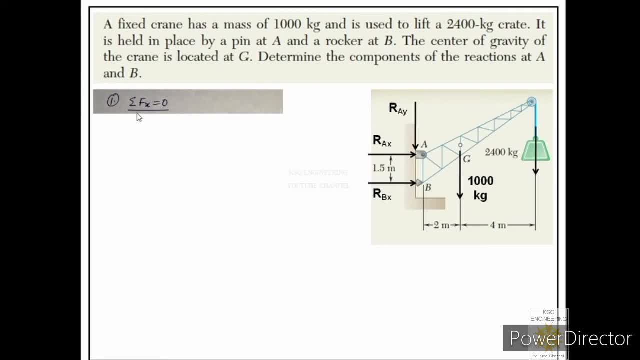 to find. so first of all, let us apply summation: FX is equal to 0. that means, as the body is in equilibrium, it means all the forces acting along X direction. their net effect must be 0. so find all the forces acting in X direction. add: 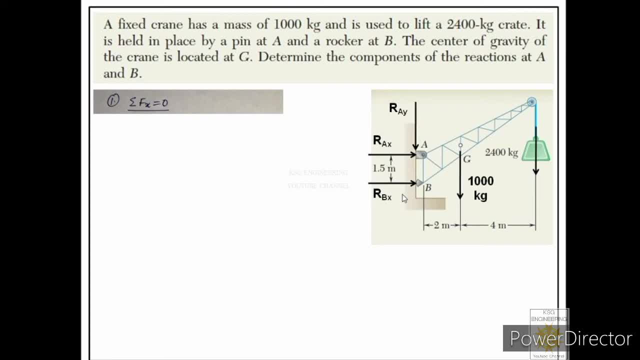 those forces and call equate those forces equal to zero. So let us see how many forces are acting in x direction. Over here you can see there are two forces acting in x direction. Then we will focus on their direction. Both are acting towards right, So both we have to consider as positive. 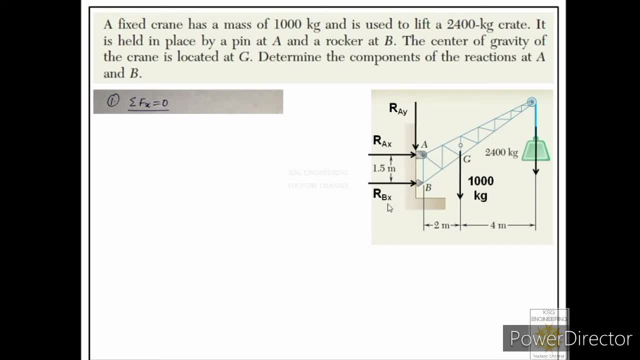 forces. So for this equation we will write: Rx plus Rbx is equal to zero. Now in this equation, both are unknown to us. So this is a single equation. we cannot solve it, So let us label this as equation 1.. Now we will apply second equation of equilibrium. 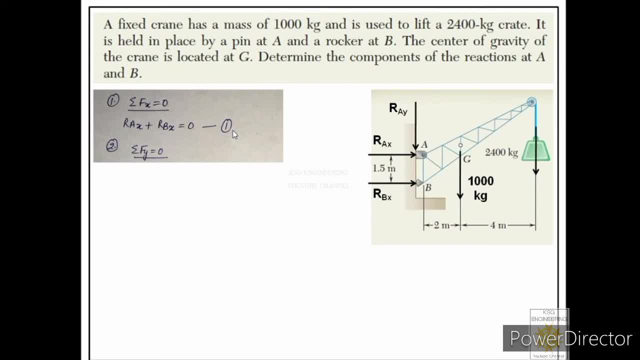 that is summation. Fy is equal to 0.. That means if the中심 Southey is in equilibrium, then all the forces acting along y direction, their sum has to be zero. so let us see how many forces are acting along y direction. add those: 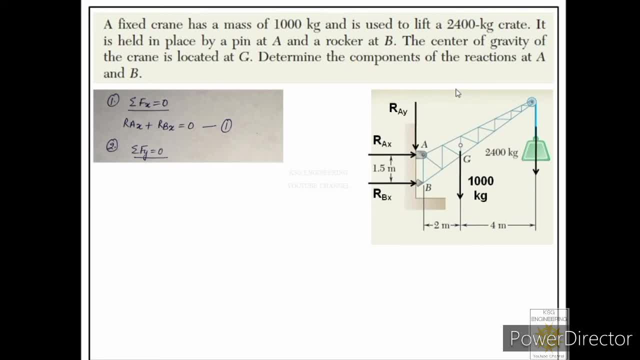 forces and equate those forces equal to zero. so you can see there are three forces acting in y direction. one is reaction RAY, second is weight of the crane, third is weight of the crate. and you can see all these three forces are acting in downward direction. so we have to consider these three negative. so let 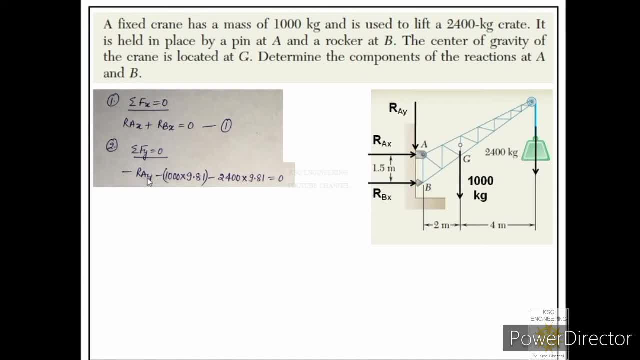 us write the equation. so equation will be: minus RAY minus 1000 into 9.81. we have converted this into weight. minus 2400 into 9.81. we have converted this also into weight is equal to zero. now in this equation, only one. 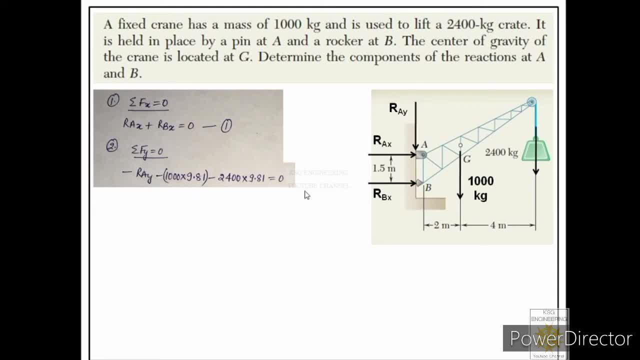 unknown is there. it means we can solve this equation. so let us solve this equation. so when you will solve this equation, you will find the value of RAY. so we have found the first answer. that is, the value of the reaction at a in y direction. now look over here. we got positive value. it means the assumption. 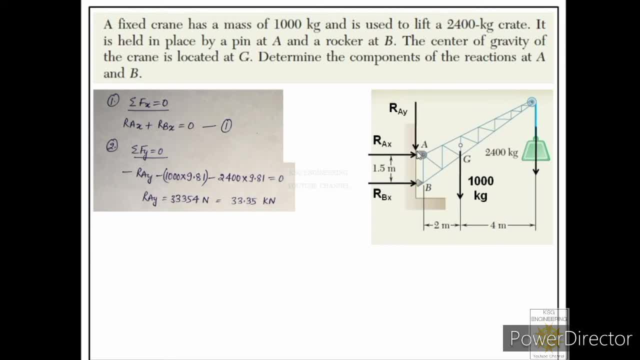 which we took at the start of the numerical is correct. it is actually acting in downward direction. now let us apply the third equation. now let us first see what is the meaning of third equation. but here we know there can be three possible displacement of a body. first is it can. 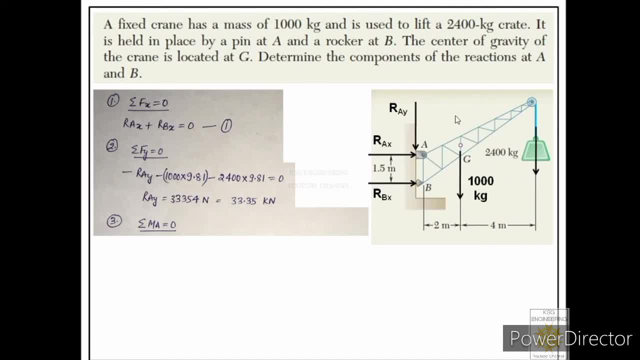 move along x direction, it can move along y direction or it can rotate. so we have used first two equations to show that it is not moving in x direction, it is not moving in y direction. now we will use third equation, that is, equation of movements, to show that body is not rotating. so how body will rotate if some 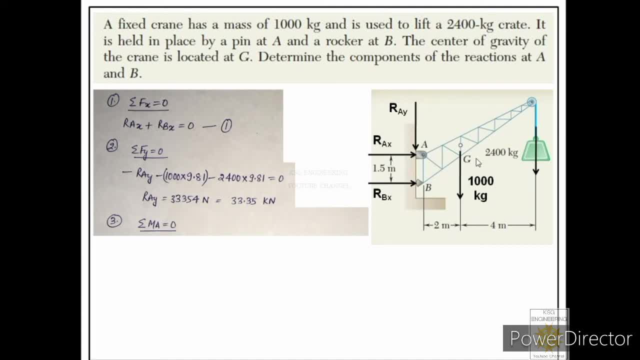 of the forces are giving movements to the body. only then body will rotate. so if the body is not rotating, that means the movements provided by the forces in the force system about any particular point must be equal to zero. so in this case we will consider a point first. at that point we will find: 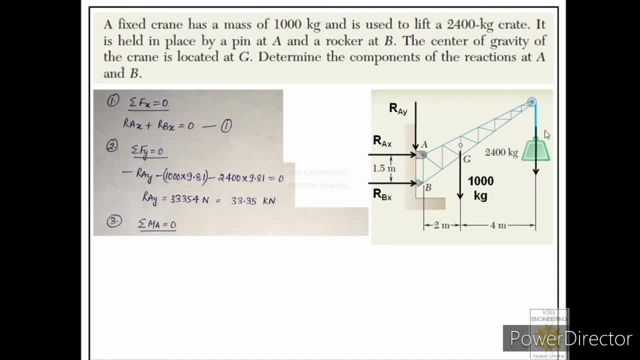 movements because of all the forces, and we will add those movements and we will equate those equal to zero, because we want to say that movement because of all the forces at any particular point is zero because body is not rotating. the next question comes, that which point we should take. 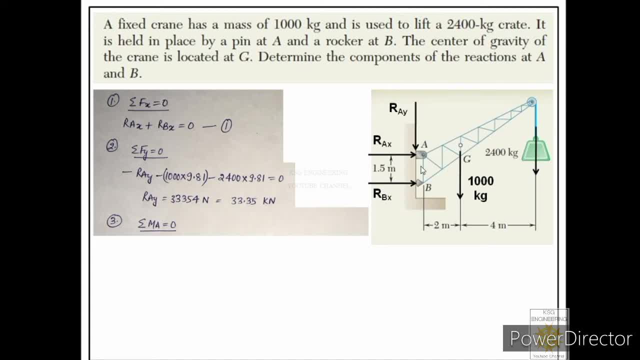 to take the movements now? answer to that question is: try to consider that point as a movement center to take the movements at which maximum forces are acting. so if you will do this, your equation will become simple. let us see how. now suppose if I take movements because of all the five forces about 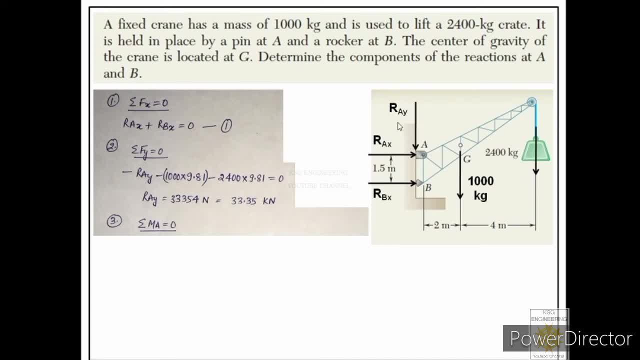 point A. then what will happen? movement because of r-a, y and r-a-x will directly become zero. why? because their perpendicular distance is zero from the movement center. so our equation will have only three moments: movements because of r-b-xmovement, because of weight of the 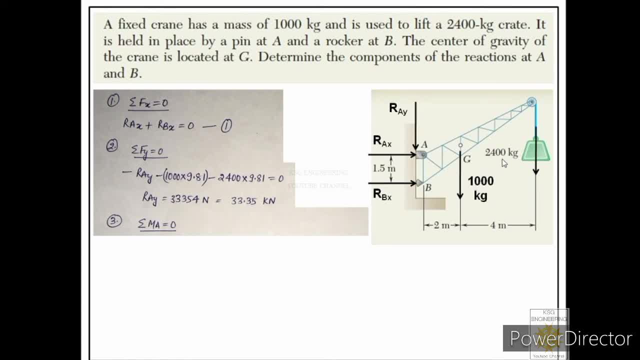 crane and movement because of weight of the crate. so our equation will become simple. but if we consider moment, let us say a point G, only movement because of the weight of the crane will be zero, but we have to calculate movement for all the other four forces. so again, I am repeating: 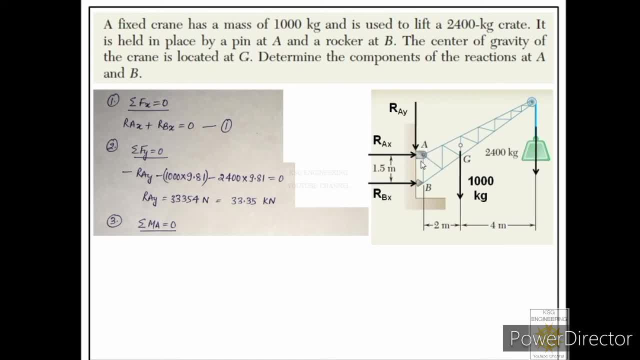 consider that point on the free body to take the moment at which maximum forces are affecting. so that is why I have written over here: movement about point A is equal to zero. so you see these two forces are directly acting at Point A, so movement because of these two will be zero. so we have to just calculate. 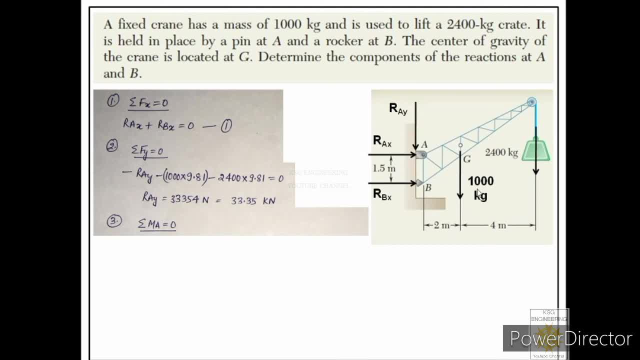 movement because of these three forces only. so let us understand movement because of RBX first at point A. now, in order to find the movement of RBX at point A, we have to first find its moment arm. so how you can find moment arm? first of all we have to find the moment arm. first of all we have to find the moment arm. 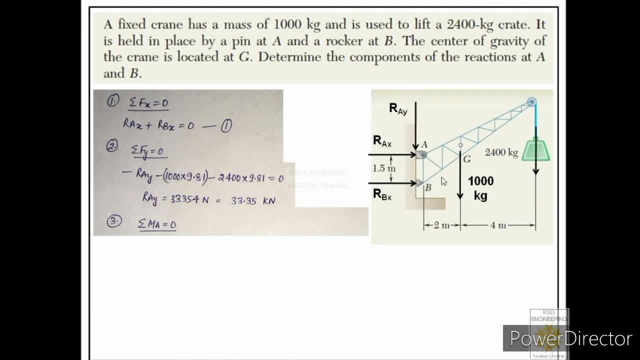 all you will locate its line of action. then from movement center you will draw a perpendicular onto that line of action. so this is the movement arm for RBX, and this movement arm is mentioned here as 1.5 meters. so for RBX movement arm is 1.5. 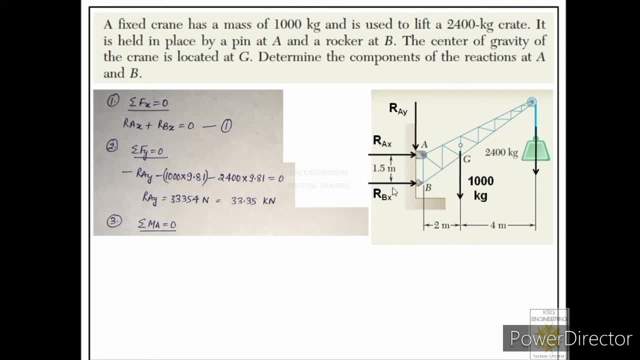 meters. next we will see what is the nature of the movement generated by this force. now you can see the shortest path between the vector and the movement center. is this only? it means, in this process, what will happen? it will generate anti-clockwise movement. so anti-clockwise movements are positive. it. 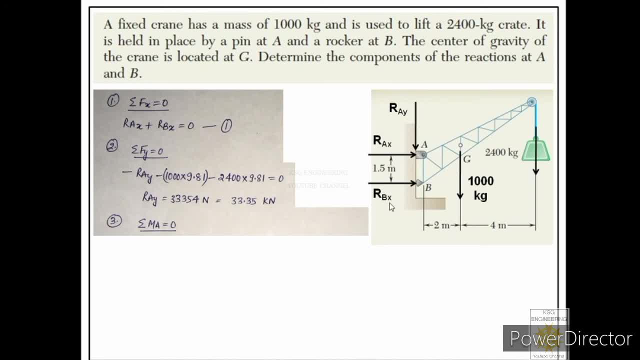 means movement because of RBX will be RBX x 1.5. now let us consider movement because of the weight of the crane. so first of all we have to find its movement arm. how to find the movement arm? now draw the line of action. now draw the line of action. 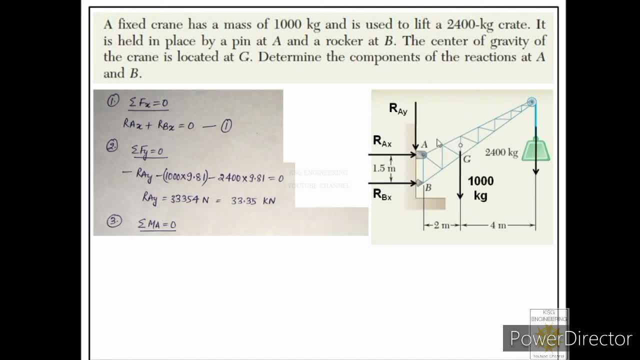 of the force and from moment center drop a perpendicular onto that force. so this moment arm is represented here as 2 meters. next we will see its nature of moment. now you can see the shortest path. is this only so vector will try to move towards the moment center, so in that process it will generate clockwise. 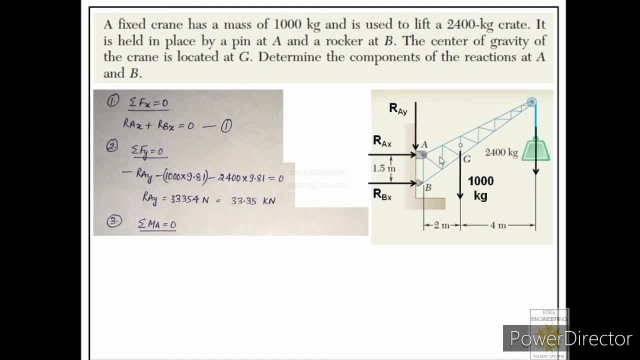 movement. fine, clockwise movements are negative. it means movement because of this weight will be minus thousand into nine, point eight, one into moment, arm, two meters. next let us see movement because of the weight of the crate. now let us first find the movement arm. so this is the line of action of that force. 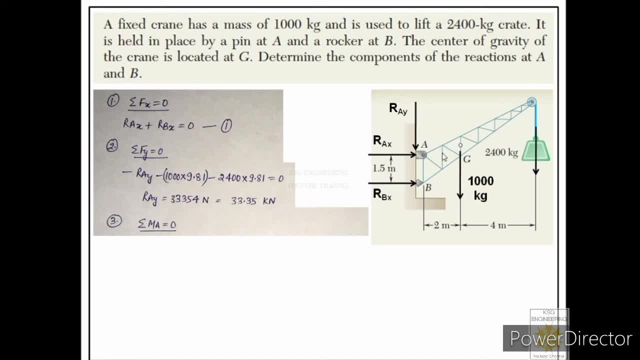 you can see that the force is moving towards the moment center. so this is the line of action of that force. so this is the line of action of that force, and from moment center drop a perpendicular onto that line of action. so this movement arm is represented here. it is equal to four plus two. that is a.